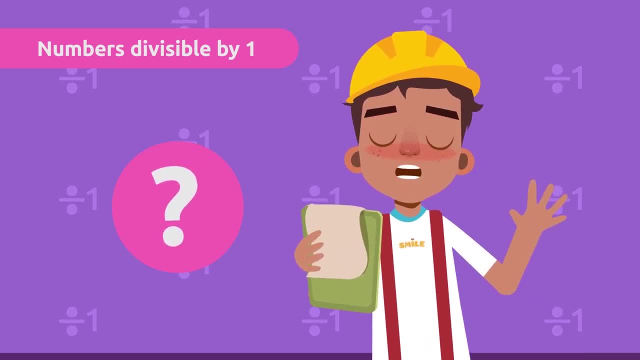 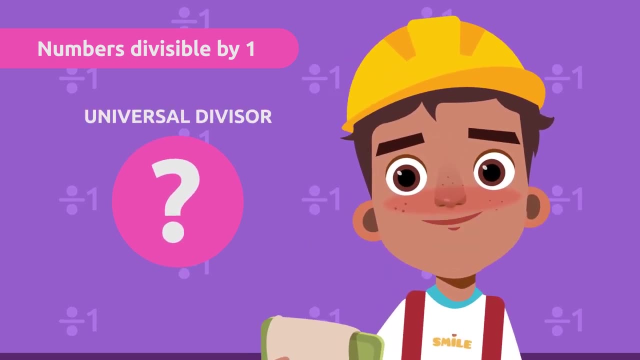 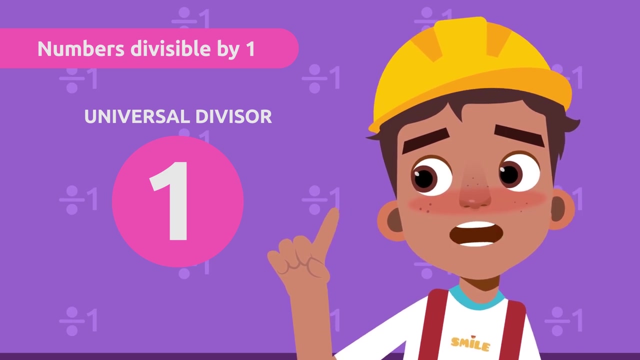 There's a very special number which no divisibility rule is needed, because any number you can think of is divisible by it. It's known as the universal divisor. Can you tell me what it is Correct? the number one: Every number can be divided by one and the remainder will always be zero. 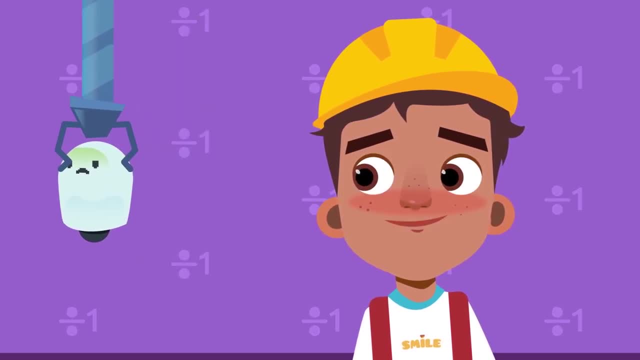 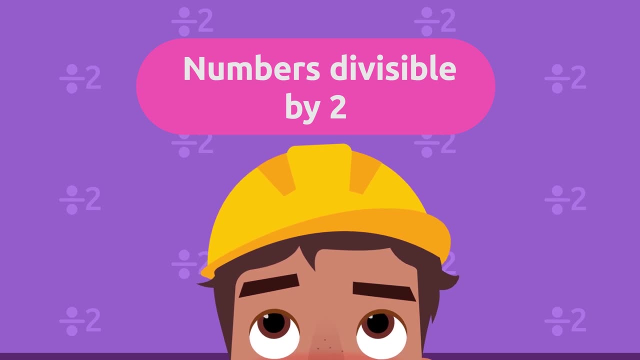 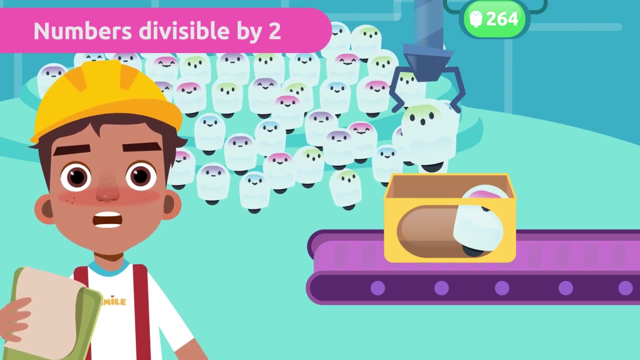 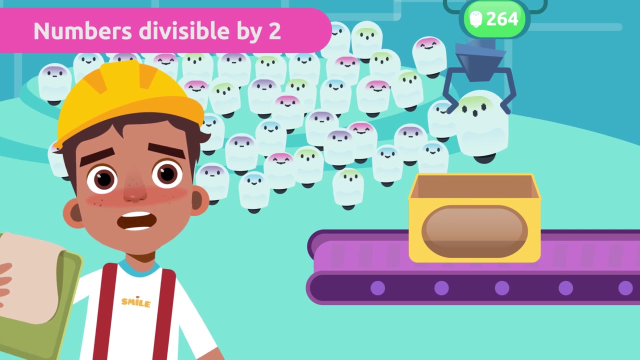 Alright, let's go solve our robot problem. Numbers divisible by two. As you see, there are 264 robots and, as I told you before that I'd want to divide by two, two, five and ten. We need to know if all the boxes will be full or if there will be robots left over. 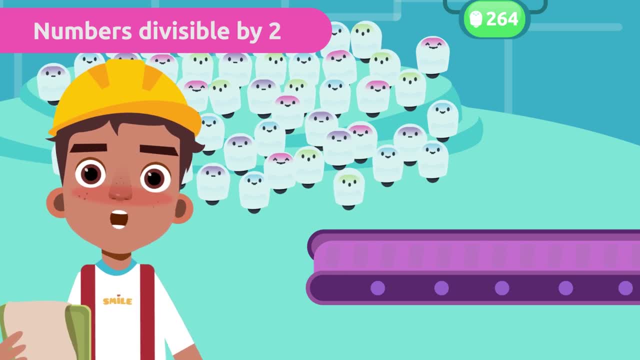 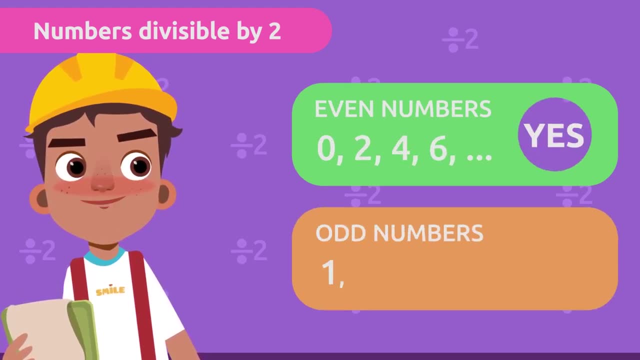 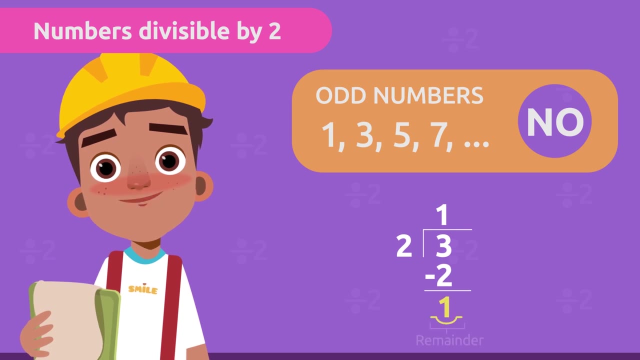 It's very easy to figure out. We can use the divisibility rule of two. If it's an even number, it's divisible by two, and if it's an odd number, it isn't divisible by two. The remainder is one, which is the number of robots left over. 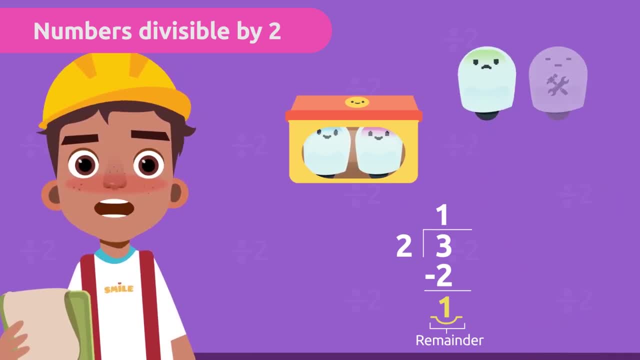 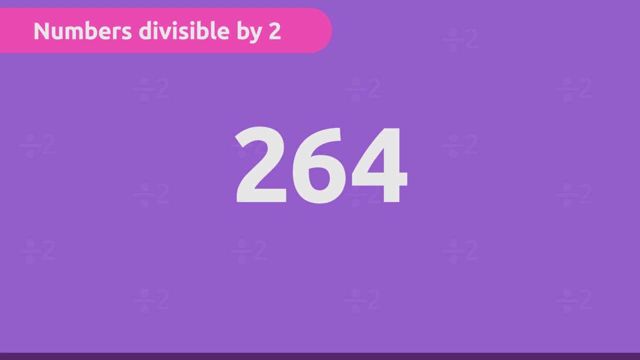 That means we will have one robot left over and we would have to make one more to fill the box. Let's give it a try To figure out if a number is odd, or even we have to look at its last digit. The last digit of 264 is four, which is an even number. 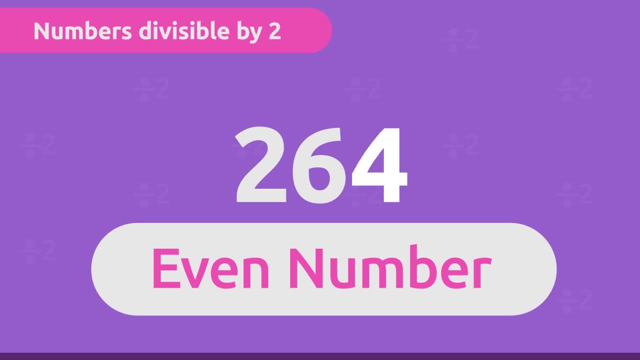 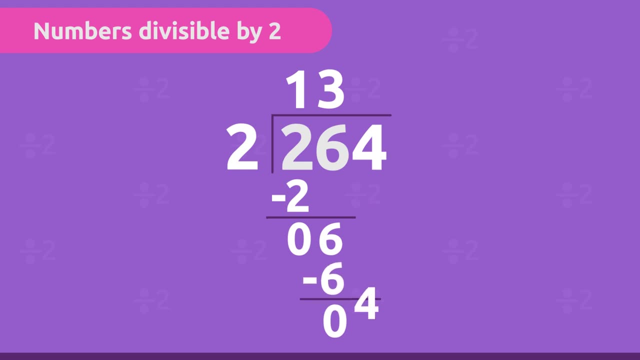 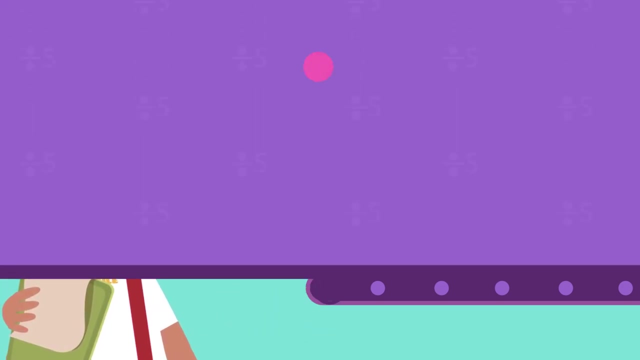 So 264 is even and it should be divisible by two. Let's test the rule. Look, The remainder is zero and we have proven that the divisibility rule of two works. Fantastic, No robot was left over. Numbers divisible by five. 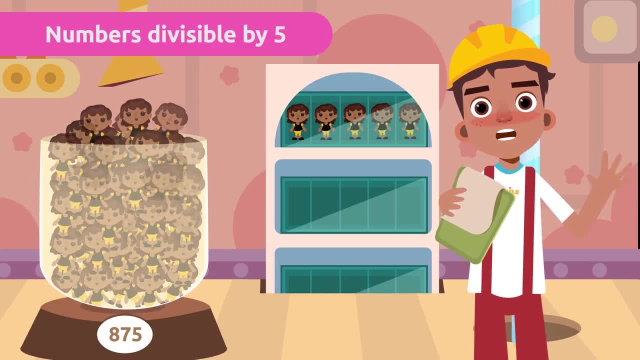 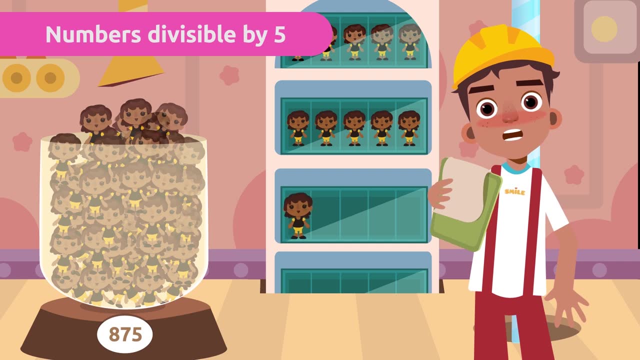 Here we have dolls. In this case, we can always keep five in each box. To find out if we can divide them into boxes of five, we use the divisibility rule of two. Let's try it. To find out if a whole number is divisible by five, we only have to look at the last digit. 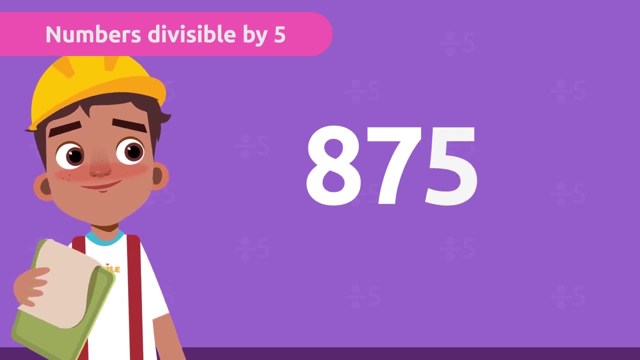 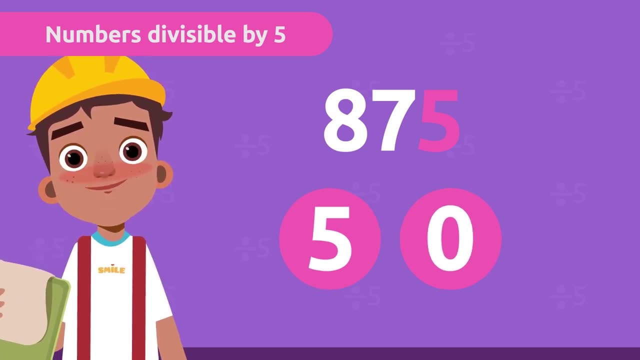 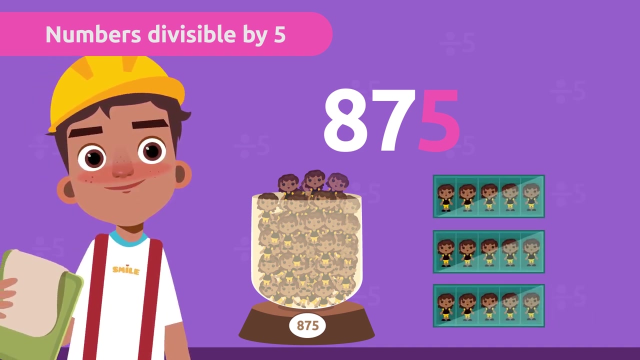 It's super easy. Every number ending in five or zero is divisible by five. There are 875 dolls, so if we store them five by five, there will be none left over. You know why? Think of the multiplication table of five.